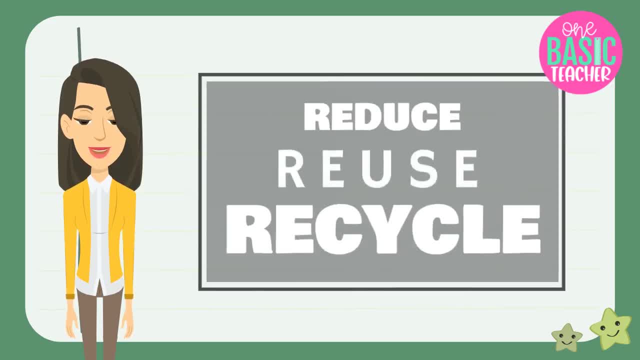 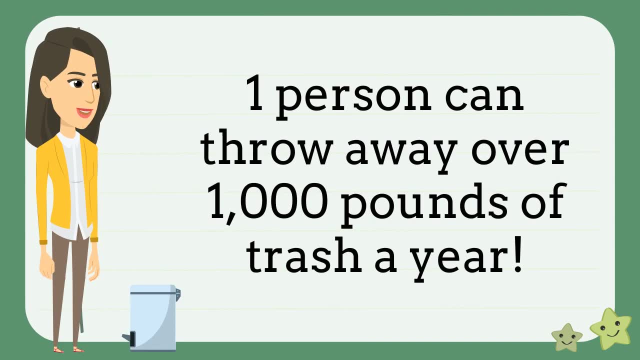 In this episode, we are going to learn how to reduce, reuse and recycle. Did you know that one person can throw away over 1,000 pounds of trash a year? That's a lot of waste and it doesn't help our planet. 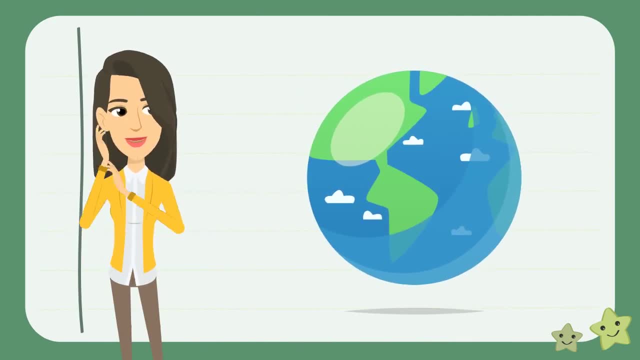 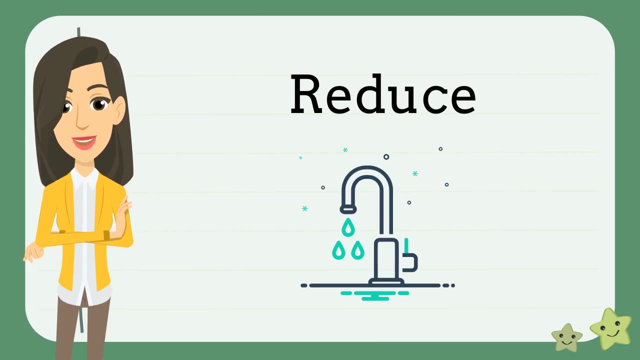 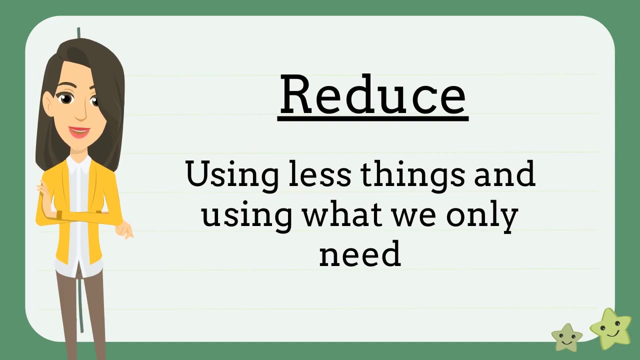 So what are some ways you can think of to help our planet? The first thing we can do is reduce waste. When we reduce waste, we are cutting down or making something smaller. When we reduce, we are using less things and using only what we need. 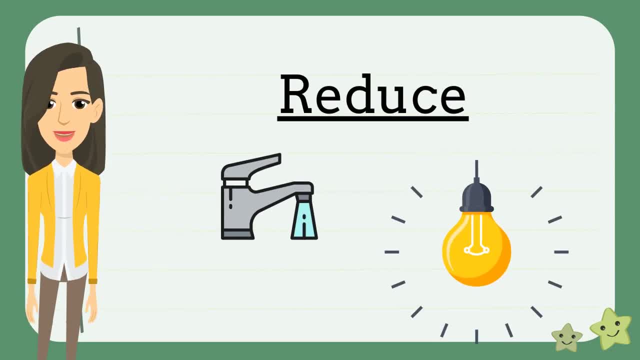 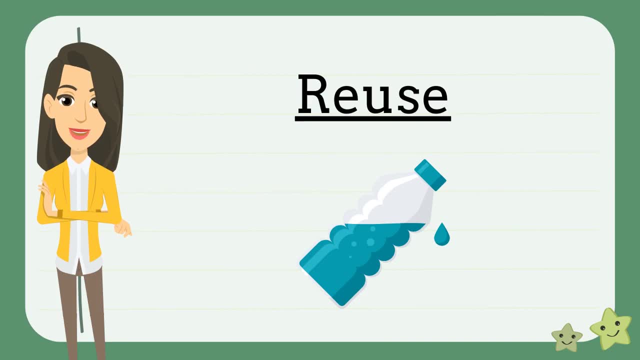 Examples of reducing are turning off the water when we are brushing our teeth and turning off the lights when we leave a room. The next thing we can do to help the Earth is to reuse things. When you reuse something, you use it again and again. 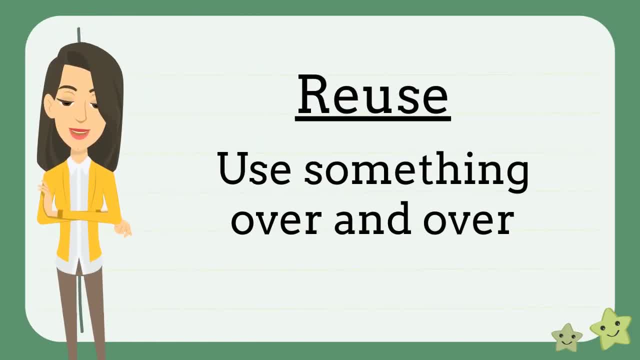 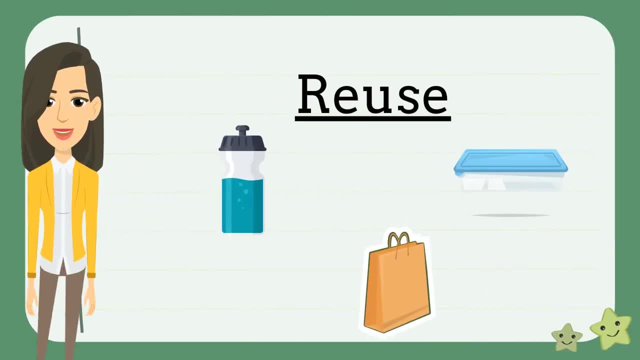 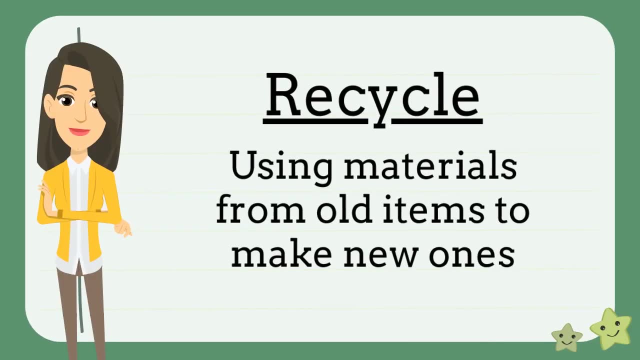 It is much better for the Earth when you reuse things over and over again. Examples of things you can reuse are lunch boxes, grocery bags and even containers. The final thing we can do to help the Earth is to recycle things. Recycling means using materials from old items to make new ones. 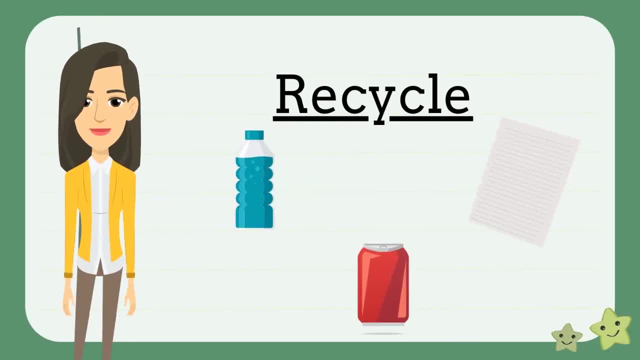 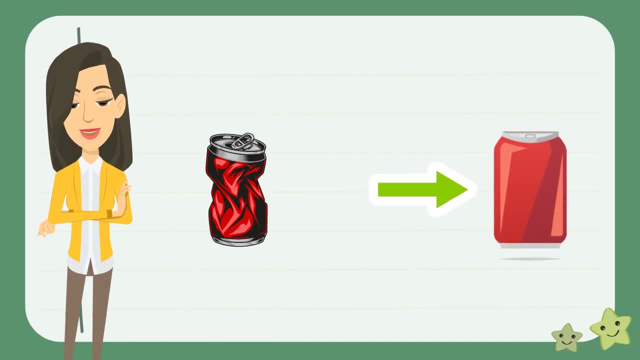 Examples of things you can recycle are plastic bottles, aluminum cans and paper. Aluminum cans can be recycled to make new aluminum cans. Plastic bottles can be recycled and turned into things such as playground equipment. Now that we've learned about the three R's- reducing, reusing and recycling- 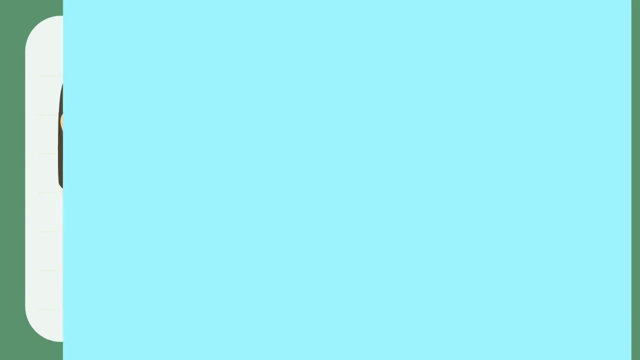 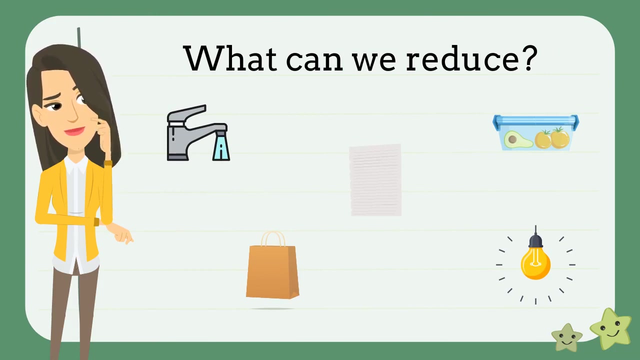 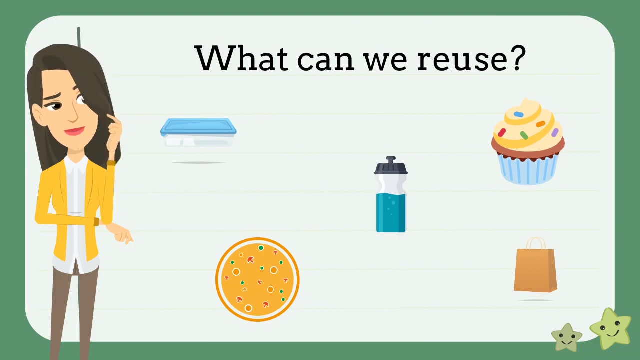 let's see if you can answer these questions. What items here can you reduce your usage of? That's right. We can reduce water and electricity by turning it off when we're not using it. Hmm, what items here can we reuse? That's right, You can reuse containers, water bottles and bags.